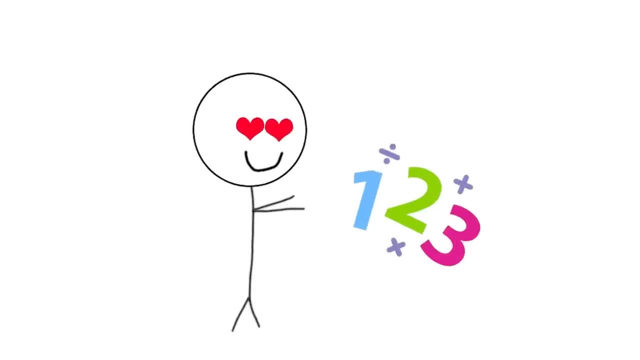 You know, as a kid I used to like math a lot. I liked it so much that I used to do it during my free time And I was on my way to becoming the Jimmy Neutron, the Phineas and Ferb, you know. 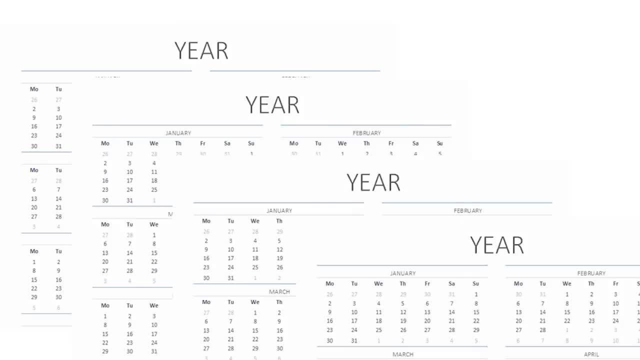 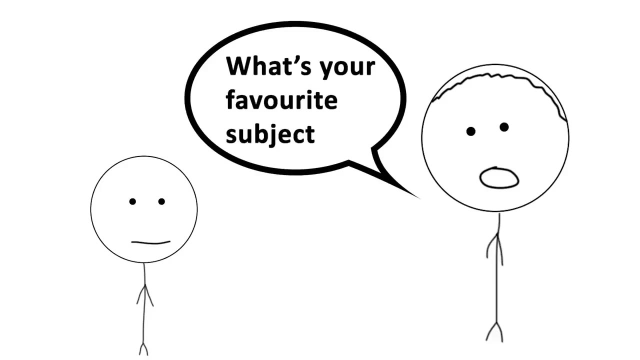 the smart characters in TV shows And for consecutive years, like a dog who sticks by its owner. I was loyal to math. My answer to the question asked most during school- what's your favorite subject- has always been, without fail, math, But after a while. 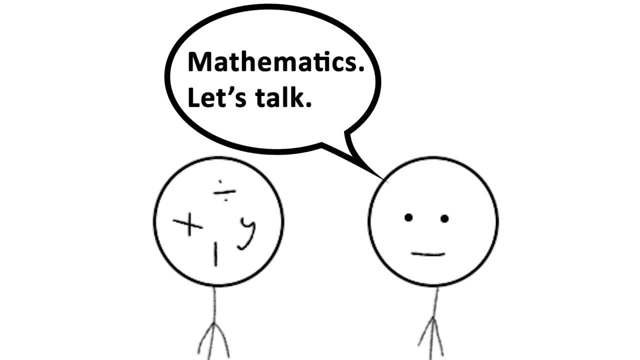 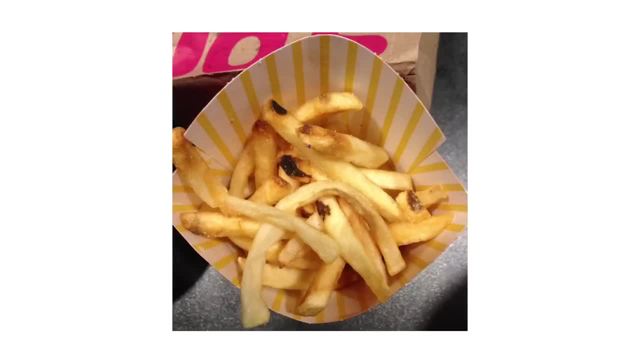 after the honeymoon phase had worn off, we stopped calling each other cute nicknames and mathematics, and I experienced some minor hurdles And, just like McDonald's fries that had gone cold, mathematics for me had just gotten stale, going from delicious to inedible. 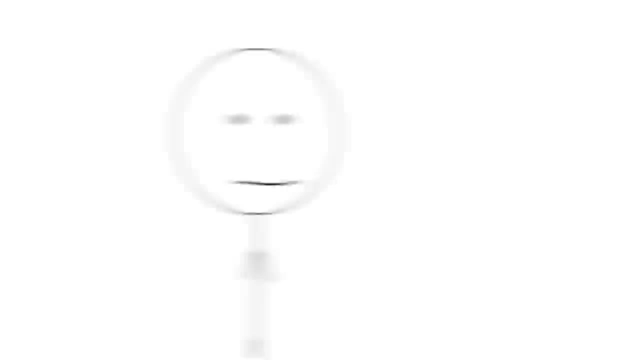 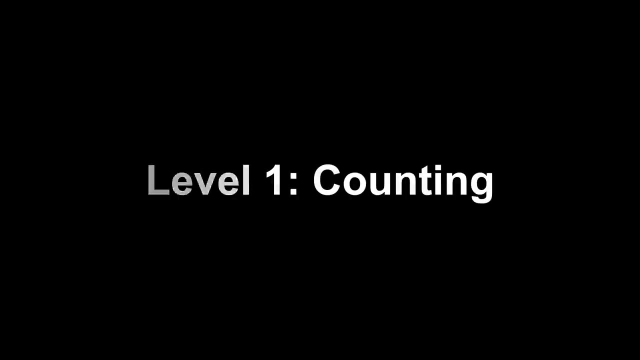 in what felt like mere moments. So I'm going to be going through the levels of mathematics I've gone through and why I've come to dislike it more and more throughout the years. Level 1. Counting: We all did it. some of us still do Counting with your fingers. 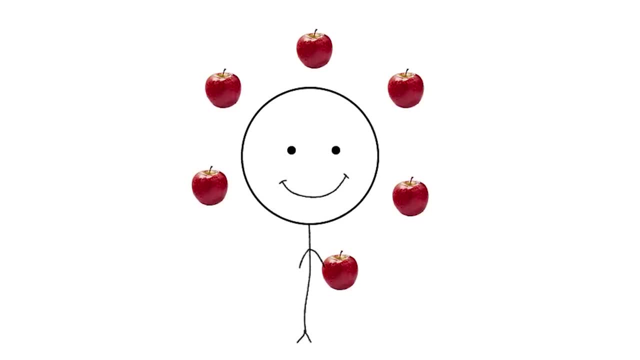 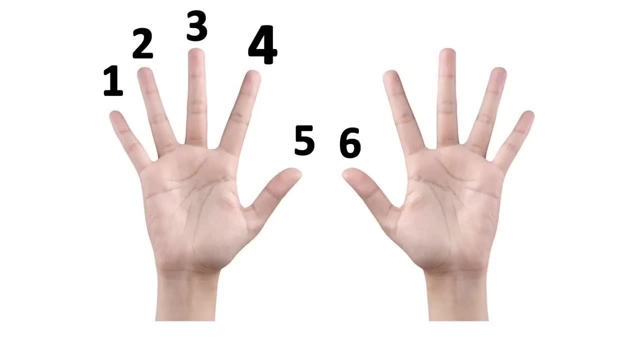 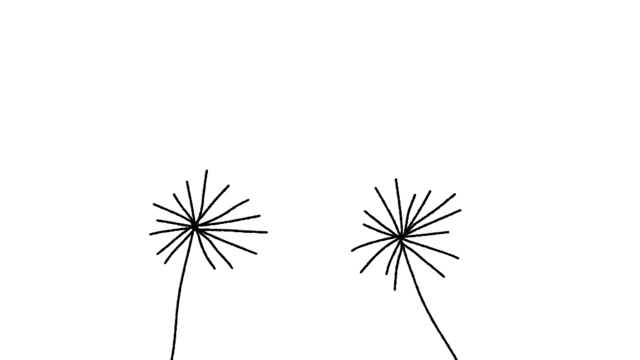 Jimmy has 4 apples and Eve gave him an extra 2.. How many apples does Jimmy have? You'd look at your fingers, start with 4, and raise 2 extra and then you count. Easy, And you might think that this will only work up to 10, because we have 10 fingers, but no, I had a way to count up to 30. 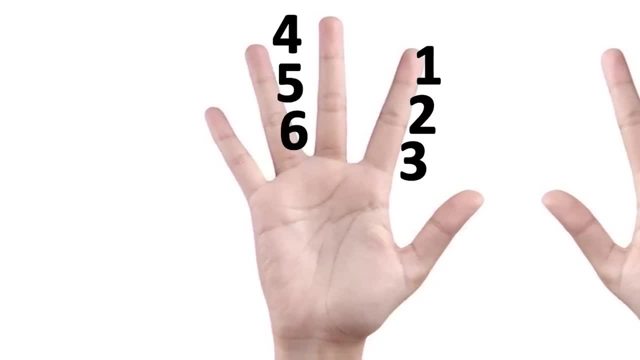 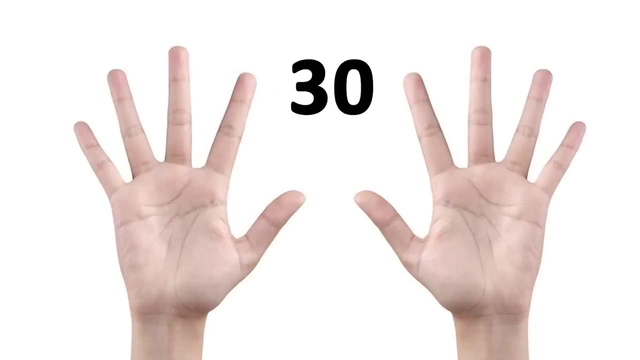 If you look at your fingers, there's 3 sections for each finger. So if you count each section instead of a full finger, you can count up to 15 numbers on each hand, And if you use both hands, it's now 30.. 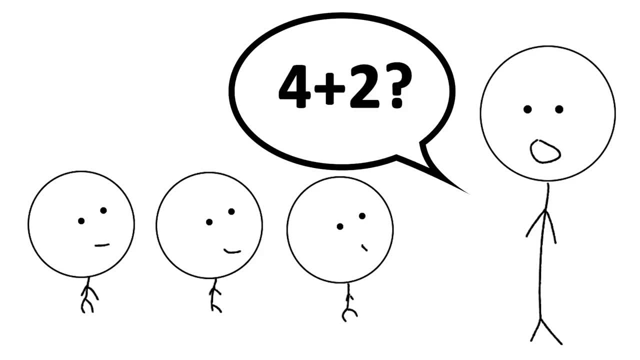 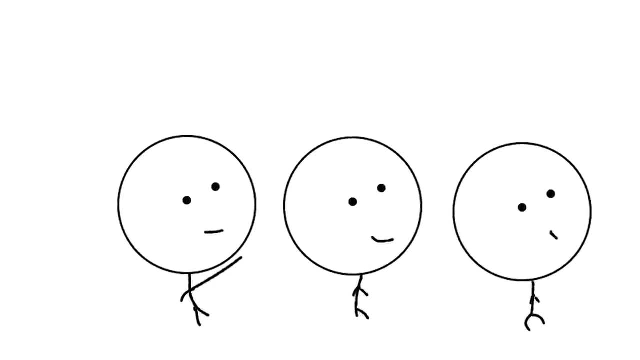 At this level of math. I remember the teacher used to ask questions at school and after a few seconds of fiddling around with our fingers or what looked like classing a spell, our arms would take off to get picked to answer the question. 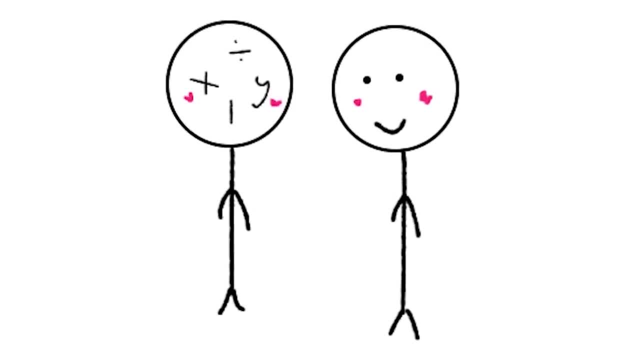 Marking the start of the relationship with math for the most of us: Level 2. Mental math. So the finger counting is only good when you're adding and subtracting less than 10 or 30 with the technique I showed, But when you get questions with bigger numbers, 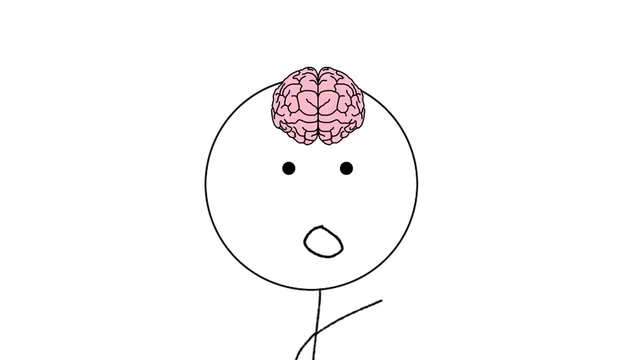 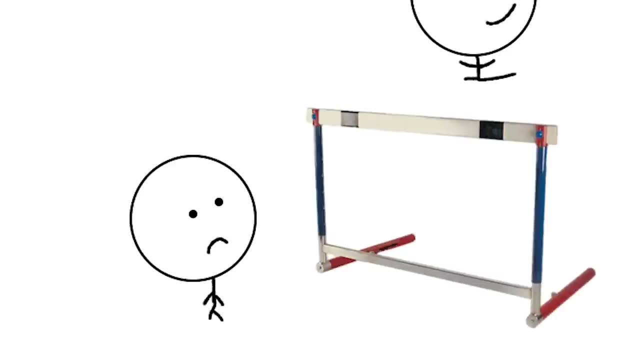 like 32 plus 12, we're forced to use our fingers to count them. So if you're not able to count, we're forced to use our brains a little bit more. This was the first big hurdle in math, where the kids who got it got it and the kids who didn't just needed more time. 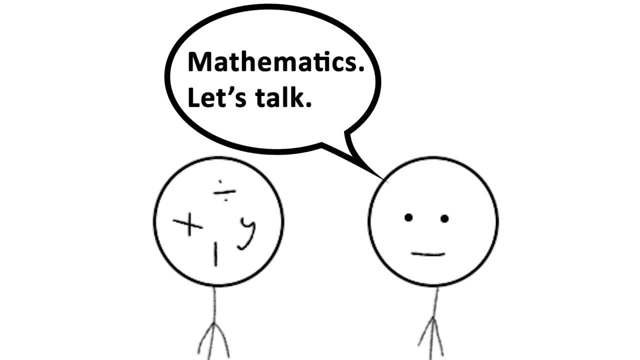 after the honeymoon phase had worn off, we stopped calling each other cute nicknames and mathematics, and I experienced some minor hurdles And, just like McDonald's fries that had gone cold, mathematics for me had just gotten stale, going from delicious to inedible. 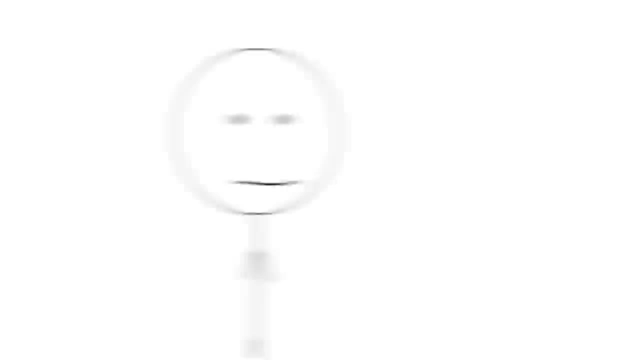 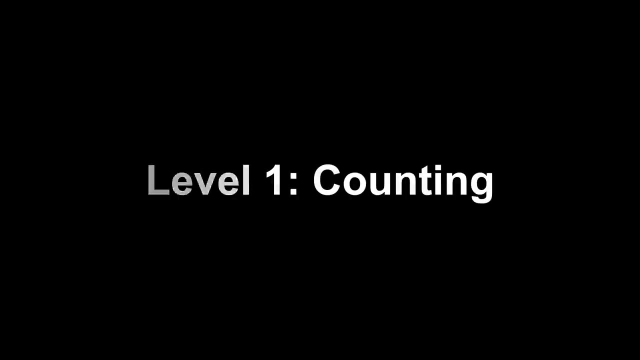 in what felt like mere moments. So I'm going to be going through the levels of mathematics I've gone through and why I've come to dislike it more and more throughout the years. Level 1. Counting: We all did it. some of us still do Counting with your fingers. 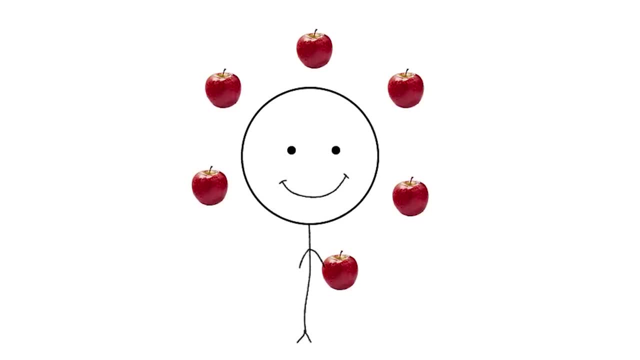 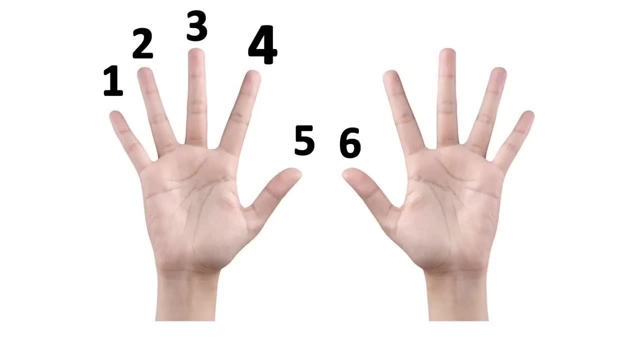 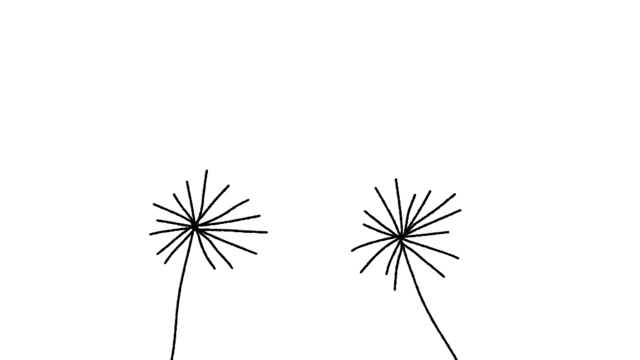 Jimmy has 4 apples and Eve gave him an extra 2.. How many apples does Jimmy have? You'd look at your fingers, start with 4, and raise 2 extra and then you count. Easy, And you might think that this will only work up to 10, because we have 10 fingers, but no, I had a way to count up to 30. 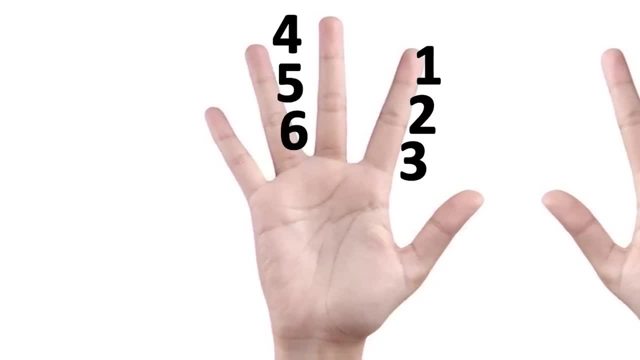 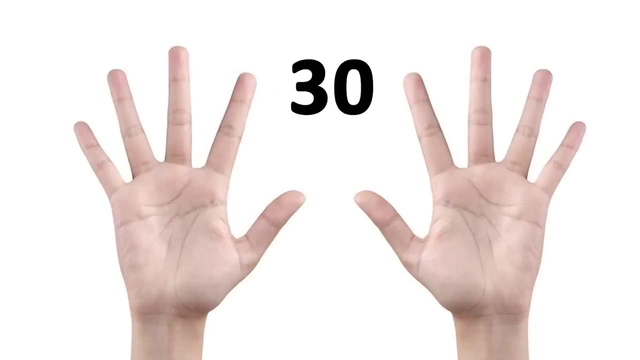 If you look at your fingers, there's 3 sections for each finger. So if you count each section instead of a full finger, you can count up to 15 numbers on each hand, And if you use both hands, it's now 30.. 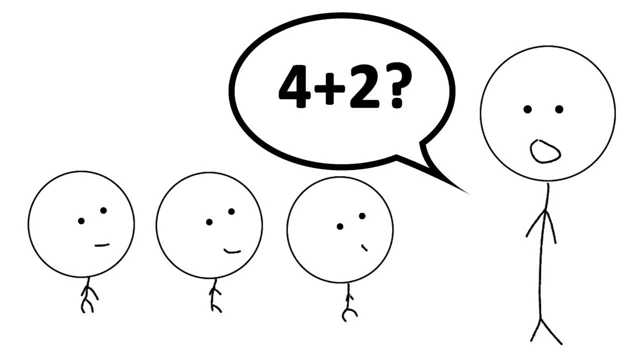 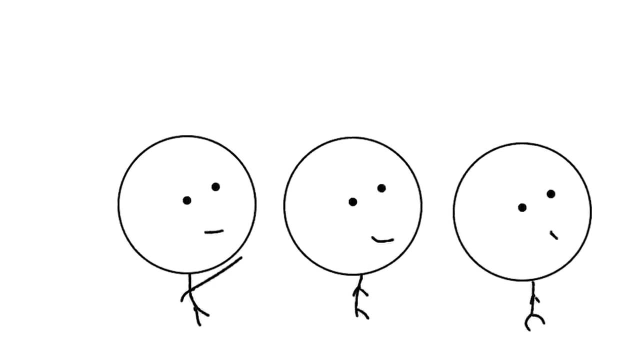 At this level of math. I remember the teacher used to ask questions at school and after a few seconds of fiddling around with our fingers, or what looked like classing a spell, our arms would take off to get picked to answer the question, marking the start of the relationship. 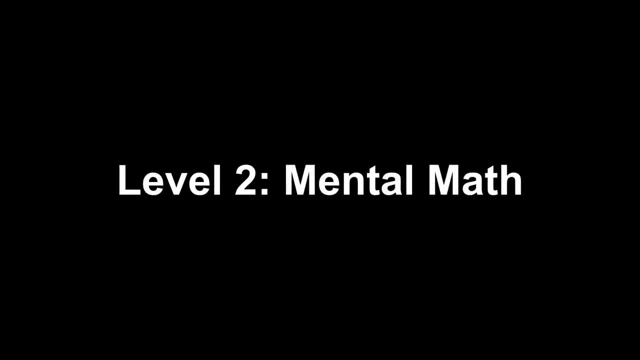 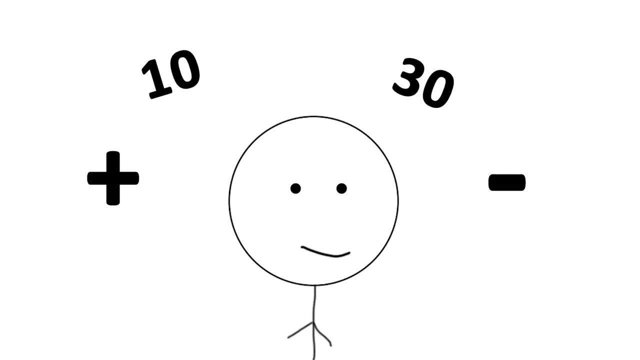 with math. for the most of us, Level 2. Mental math. So the finger counting is only good when you're adding and subtracting things less than 10 or 30 with the technique I showed, But when you get questions with bigger numbers like 32 plus 12,. 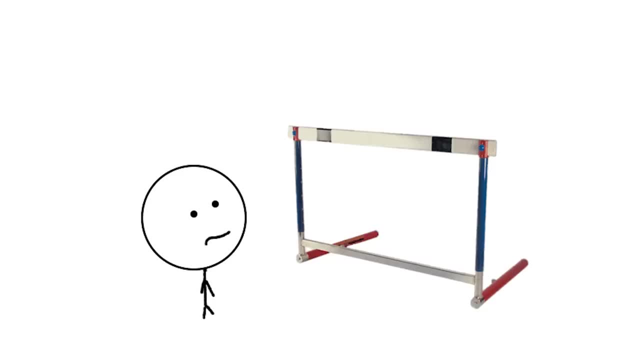 we're forced to use our brains a little bit more. This was the first big hurdle in math, where the kids who got it got it, and the kids who didn't just needed more time. Now, I was one of those kids who didn't get it when the teacher taught us. 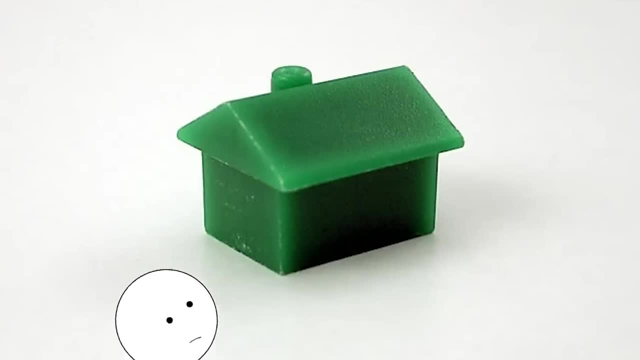 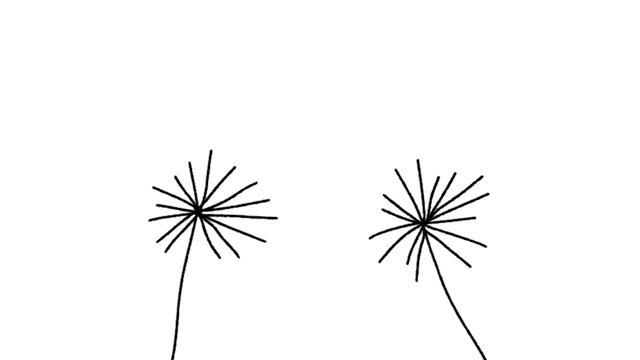 but I had a genius idea. When I got home from school that evening, I grabbed a marker and drew 50 dots on my arm. Why, you might ask. I figured I couldn't add extra fingers on myself. and even if I could, I didn't want my hands to look like a star-nosed 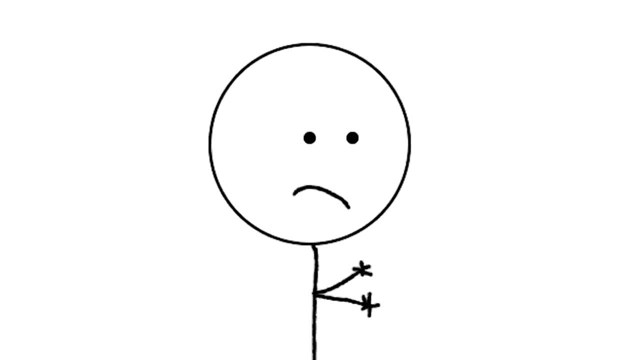 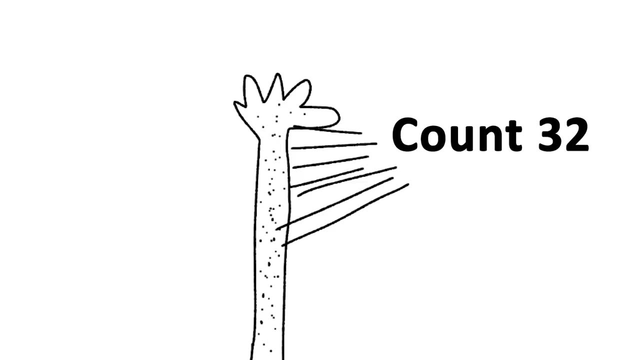 mole. I didn't want my fingers to look like a star-nosed mole. I didn't want my fingers to look like a star-nosed mole. So, to bypass this physical limitation, I thought about the idea of drawing dots on myself: 32 plus 12,. no problem, I'll count 32 dots and I'll shift my finger. 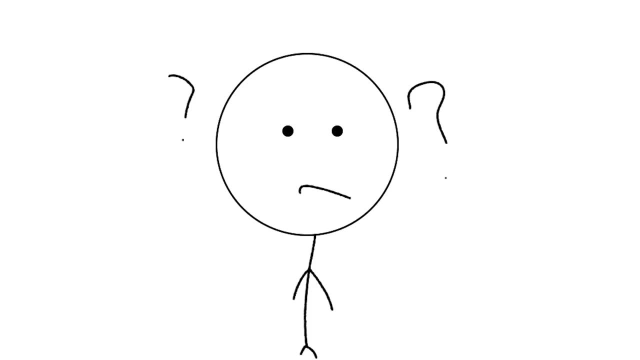 Now, I was one of those kids who didn't get it when the teacher taught us. But I had a genius idea. When I got home from school that evening, I grabbed a marker and drew 50 dots on my arm. Why, You might ask? I figured I couldn't add extra fingers on myself. 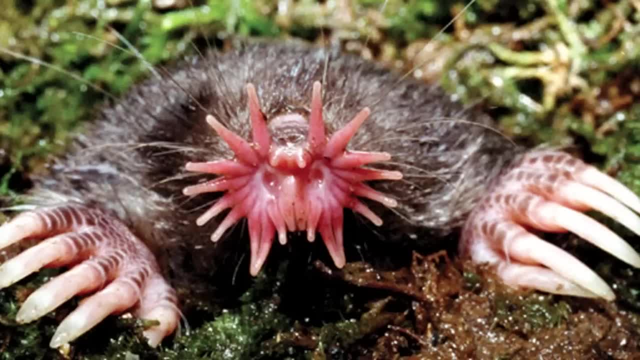 and even if I could, I didn't want my hands to look like a star-nosed mole. Level 3. Using your fingers to count numbers, So if you're not able to count them, you can't count them. Level 4. Using your fingers to count numbers, So if you're not able to count them, you can't count them. 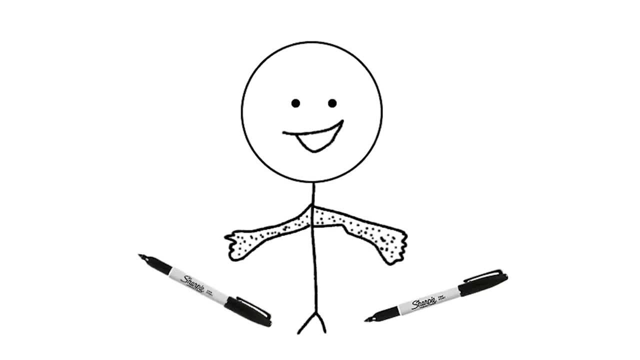 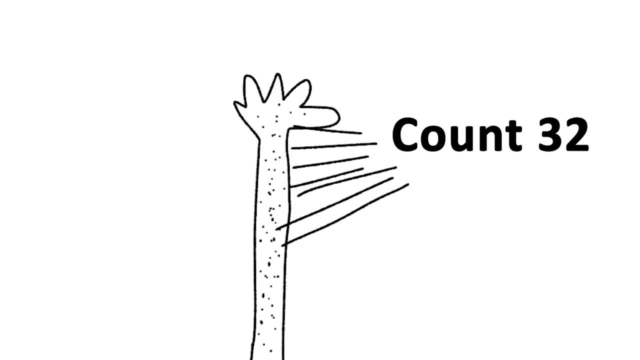 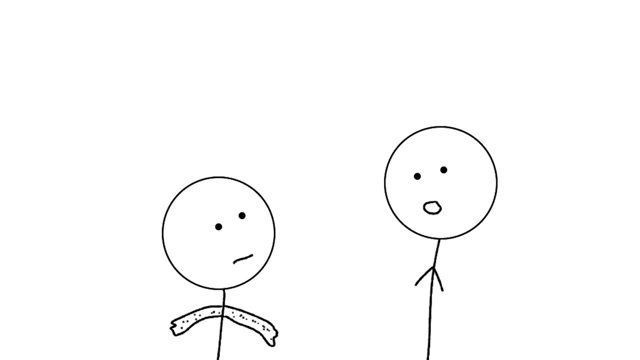 So, to bypass this physical limitation, I've thought about the idea of drawing dots on myself, 32 plus 12.. No problem, I'll count 32 dots and I'll shift my finger across my arm until I finish counting a further 12.. The only bad thing about this is that the teacher told me to wash off the 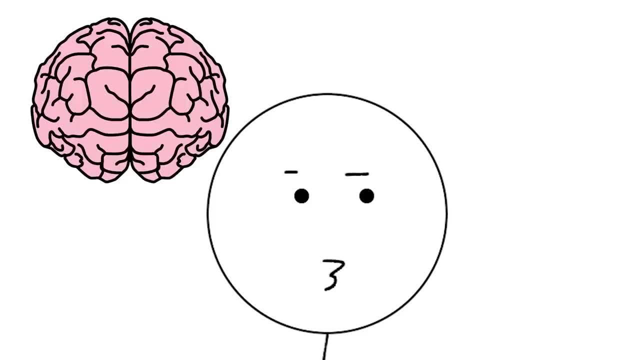 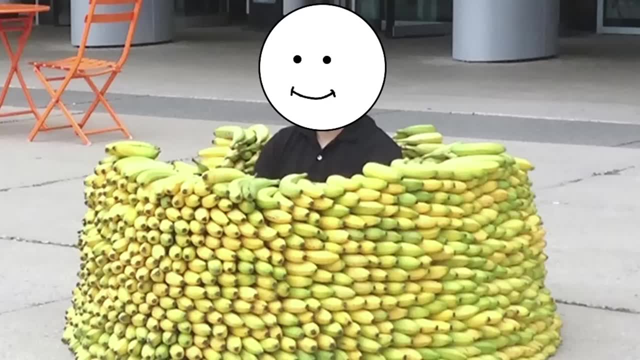 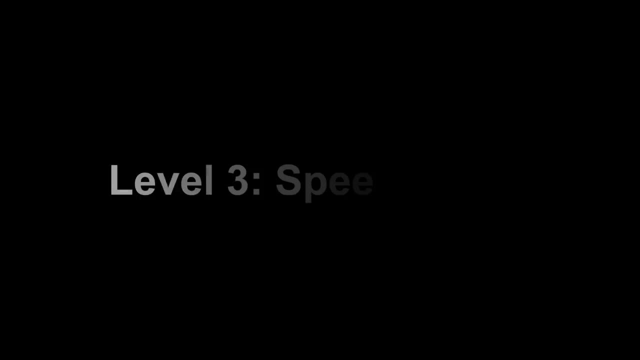 dots the next day because I guess the topic was mental math and not counting. Honestly, I think she was just jealous, But eventually I learnt how you're supposed to solve questions that didn't or couldn't have physical representations for Level 5.. Level 3. Speedy Math. 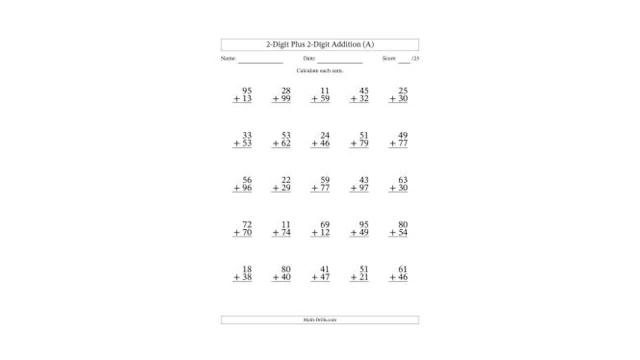 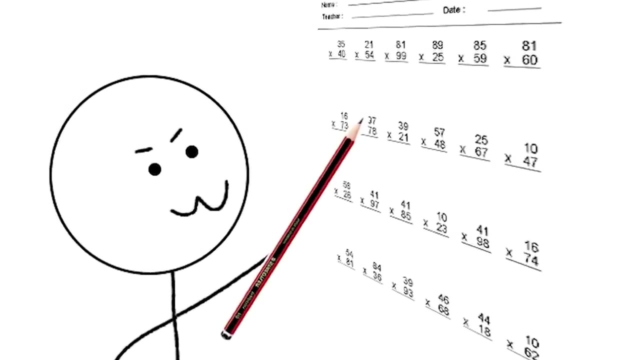 This was my favourite. Remember those math sheets we used to get with maybe 15 questions. I remember zooming through these questions and after I'd finished, the graphite from the pencil would stain the blade of my hand from signing on the pencil markings on the paper. 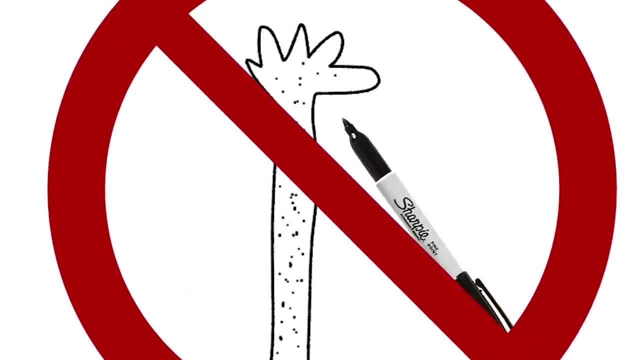 No more mental math, No more drawing dots on myself. Level 6.. Level 7.. Level 8.. Level 9.. Level 10.. Level 11.. Level 12.. I remember the teacher would give us a sheet of questions and test us every morning. 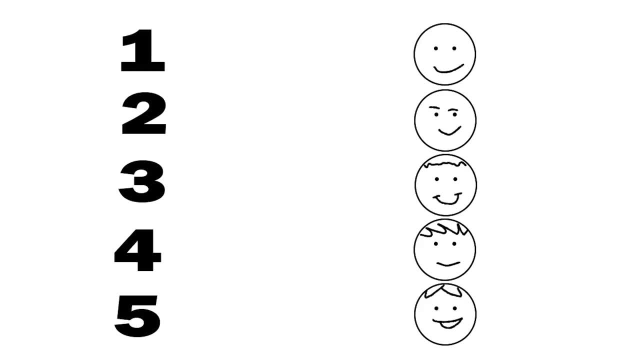 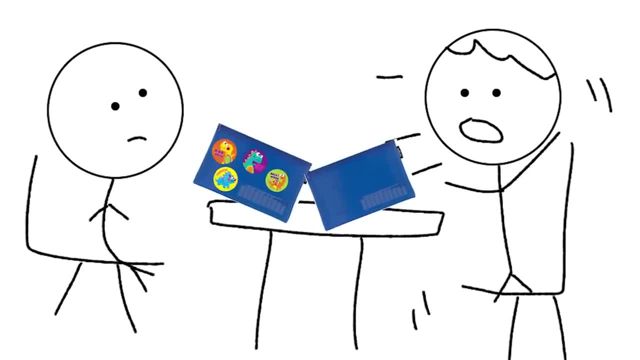 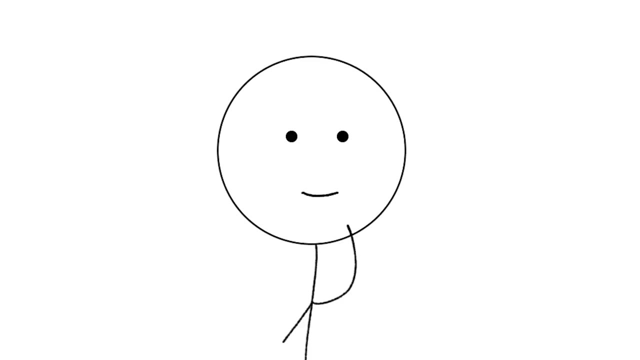 and the top 5 people to finish first with no mistakes got a sticker. I had 4 stickers on my pencil case and if someone was bothering me during class, all I had to do was ask a simple question: How many stickers do you have? Completely soul crushing. I was responsible for that annoying 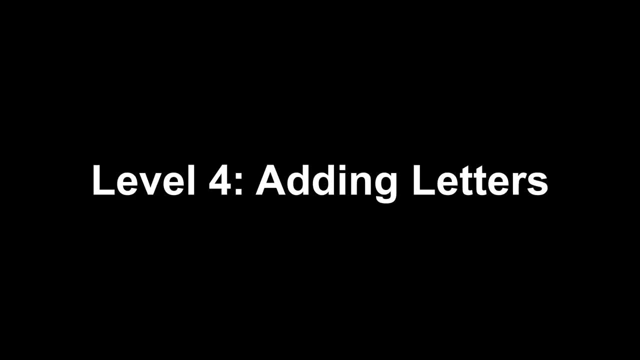 kid's childhood trauma: Level 4. Adding letters: Level 7.. Level 8.. Level 9.. Level 10.. Level 11.. Level 12.. Level 13.. Level 14., Level 15. Level 15.. 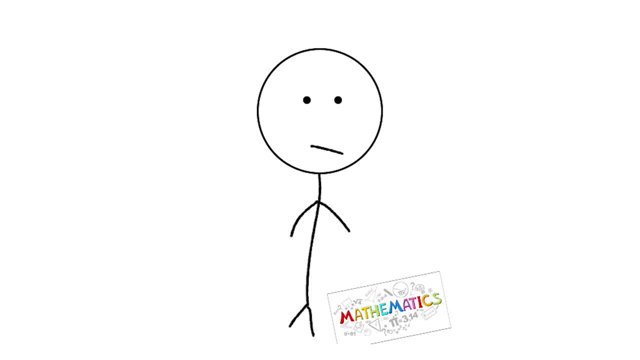 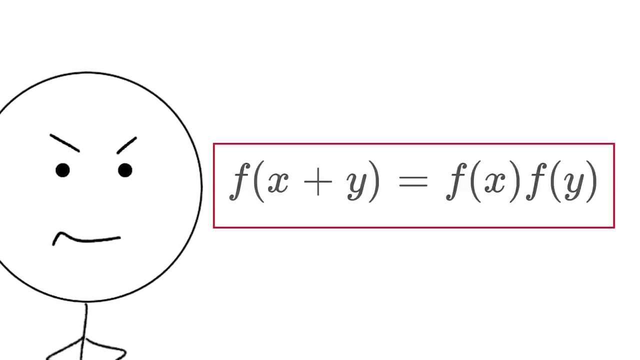 For me, my positive experience with math ends here. Level 4 marks the start of my turbulent relationship with math. My understanding was we have numbers for math and letters for English. That's how it was, But then they started adding random letters in with the numbers. 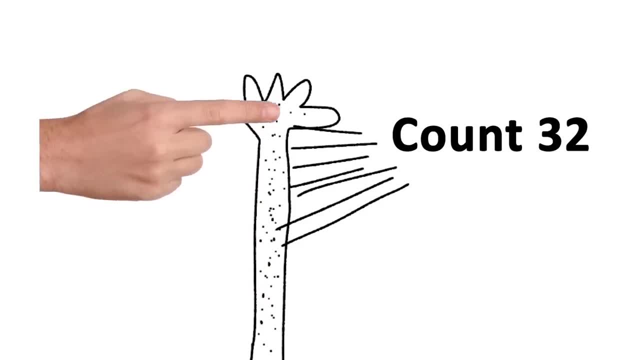 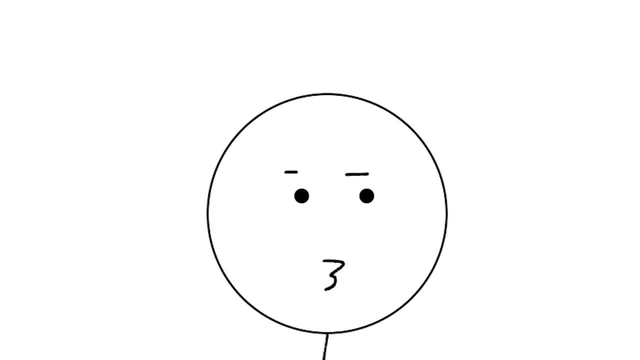 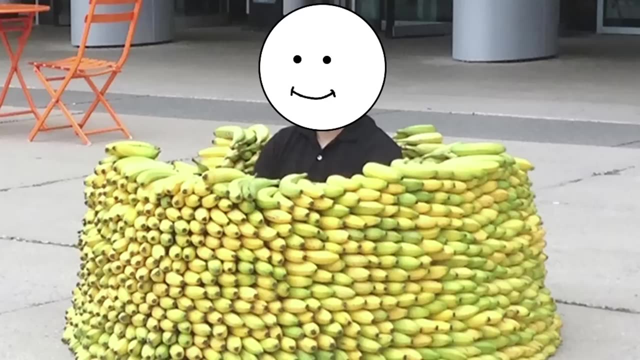 across my arm until I finish counting a further 12.. The only bad thing about this is that the teacher told me to wash off the dots the next day because I guess the topic was mental math and not counting. Honestly, I think she was just jealous, But eventually I learnt how you're. 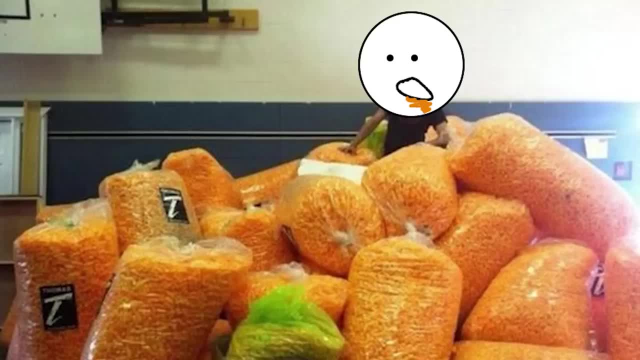 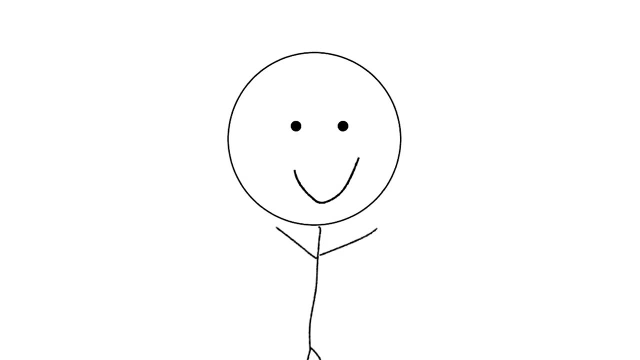 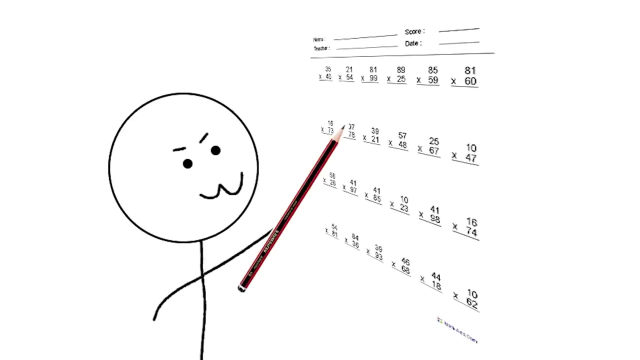 supposed to solve questions that didn't or couldn't have physical representations. for further climbing up the mountain of mathematics, Level 3. Speedy math: This was my favourite. Remember those math sheets we used to get with maybe 15 questions. I remember zooming through. 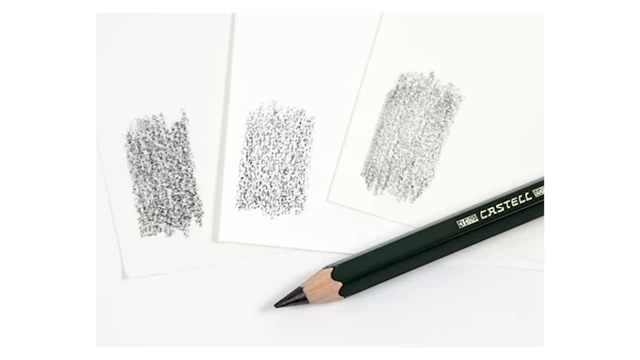 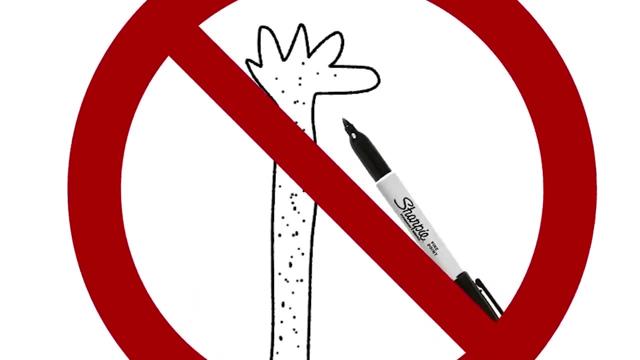 these questions and after I'd finished, the graphite from the pencil would stain the blade of my hand from signing on the pencil markings on the paper. No more mental math. No more drawing dots on myself. I remember the teacher would give us a sheet of questions and test us every. 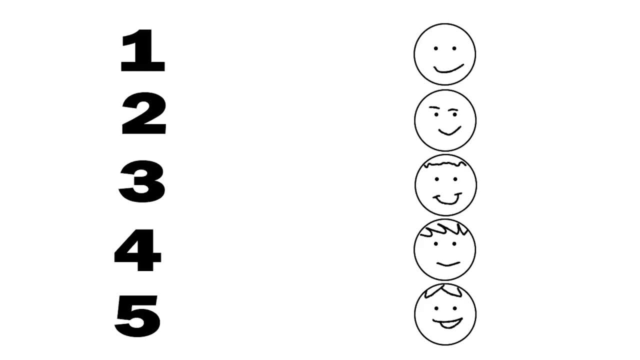 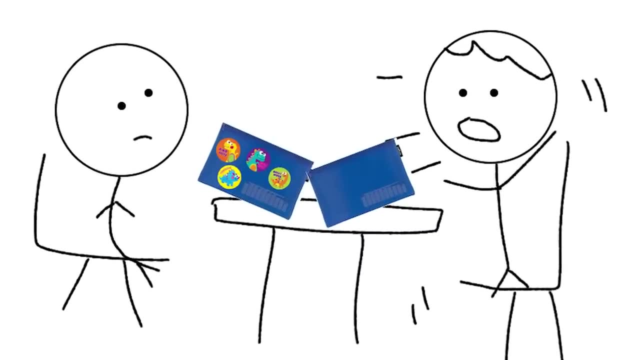 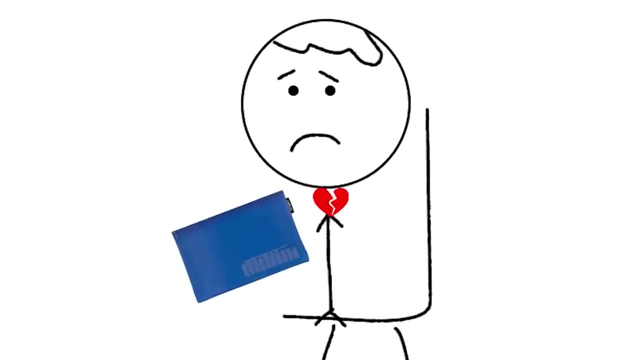 morning And the top 5 people to finish first with no mistakes got a sticker. I had 4 stickers on my pencil case and if someone was bothering me during class, all I had to do was ask a simple question: How many stickers do you have? Completely soul crushing. I was responsible for that annoying 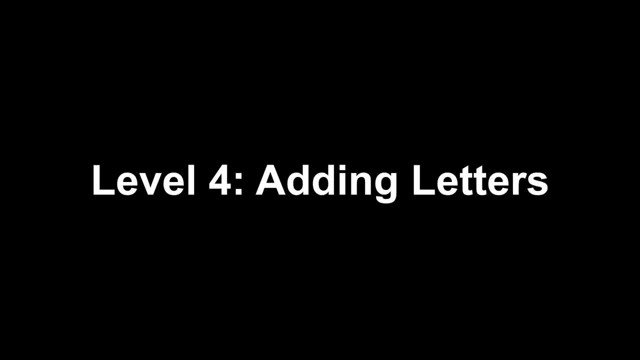 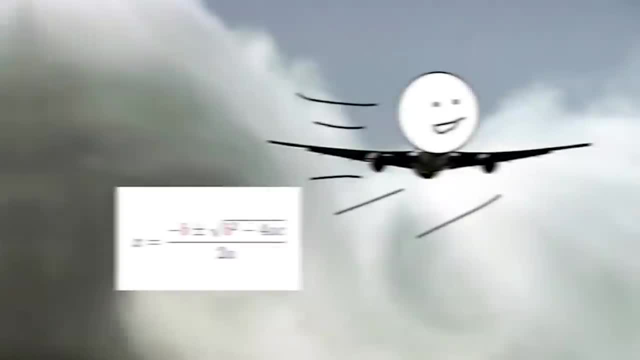 kid's childhood trauma- Level 4. Adding letters. For me, my positive experience with math ends here. Level 4 marks the start of my turbulent relationship with math. My understanding was we have numbers for math and letters for English. 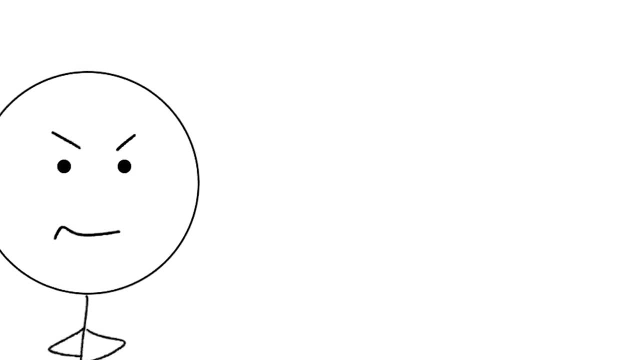 That's how it was, But then they started adding random letters in with the numbers. It started off with a couple of letters- x's and y's, But then math started bringing in more letters: N's, Z's and an E, which apparently represents a number. 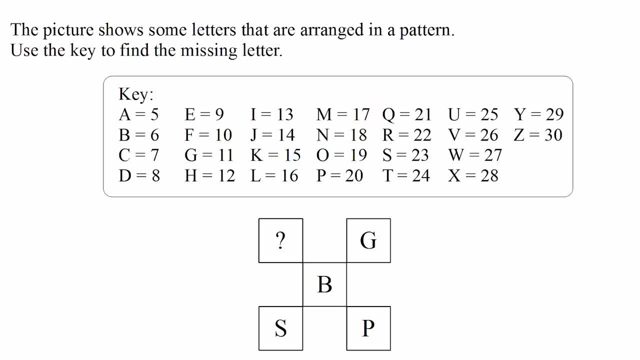 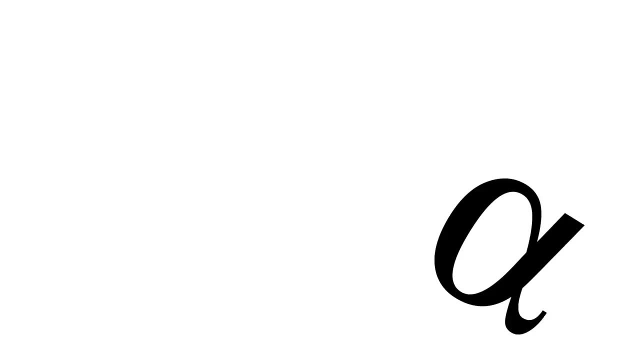 Sometimes I'd think I was in an English class because there would be so many letters and I would mistakenly answer vowel for E. But a line was crossed when they added Greek letters- Alpha, beta, theta- It was now apparently a language class as well. 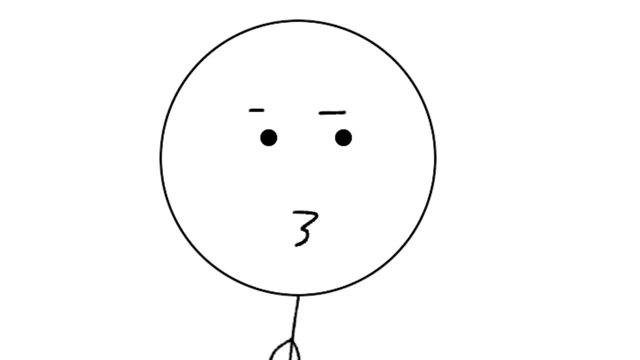 What happened to good old numbers, And I know I shouldn't compare, since comparison is often the thief of joy, But all I'm saying is that in English we didn't have to count the number of vowels and multiply it by the consonants. 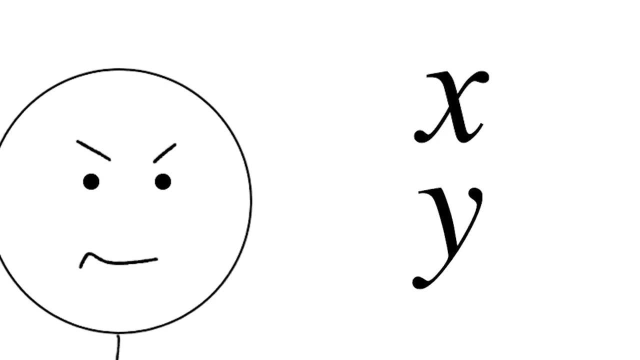 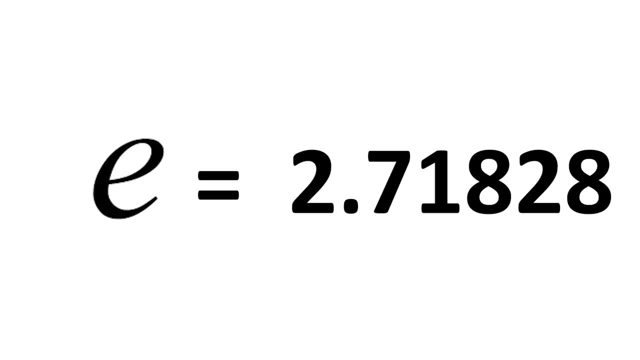 It started off with a couple of letters- Xs and Ys, But then math started bringing in more letters: Ns, Zs and an E, which apparently represents a number. Sometimes I'd think I was in an English class because there would be so many letters. 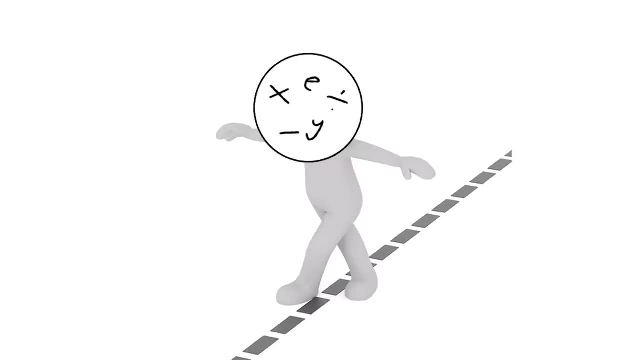 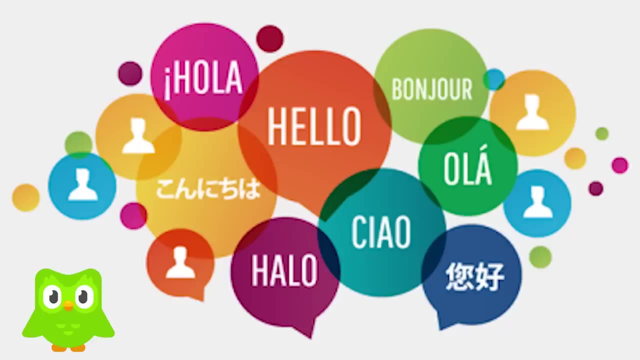 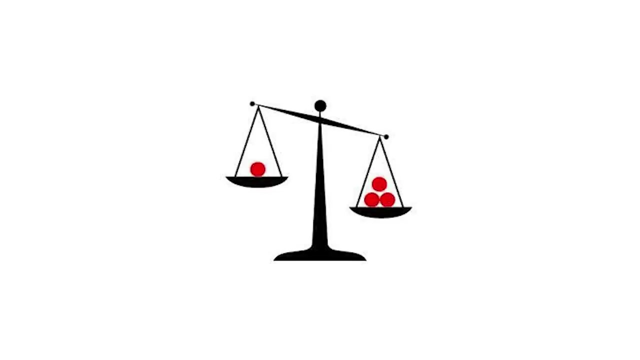 and I would mistakenly answer vowel for E, But a line was crossed when they added Greek letters- Alpha, Beta, Theta. It was now apparently a language class as well. What happened to good old numbers? And I know I shouldn't compare, since comparison is often the feat of joy, But all I'm saying 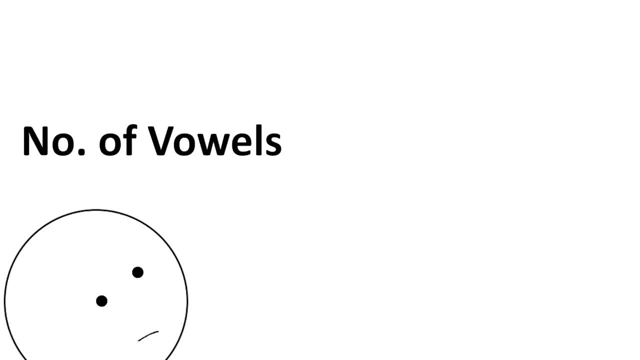 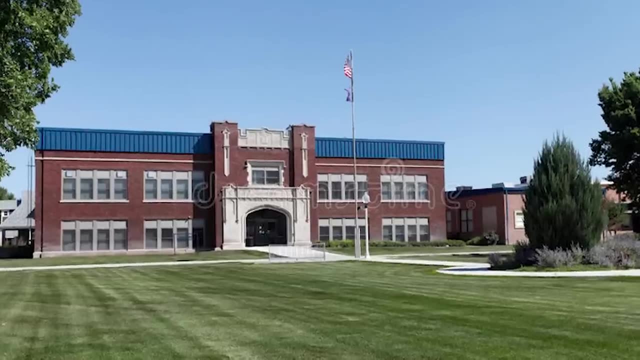 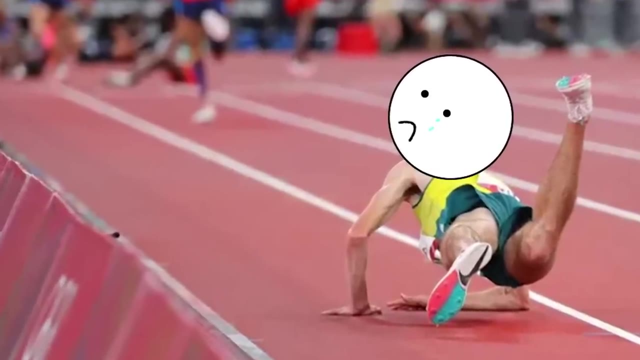 is that in English we didn't have to count the number of vowels and multiply it by the consonant Level, 5, triangles. I remember in the final stages of secondary school. if you miss a class it's game over, Just like tripping over at the start of a 100m sprint. 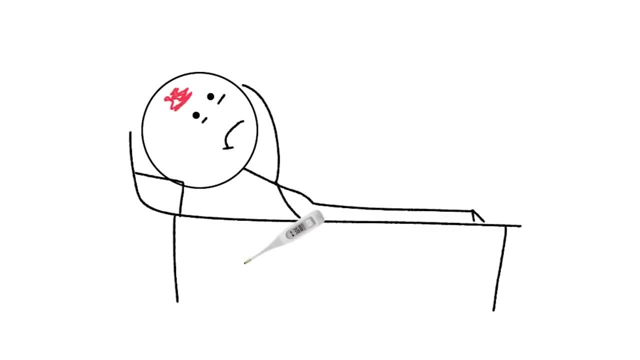 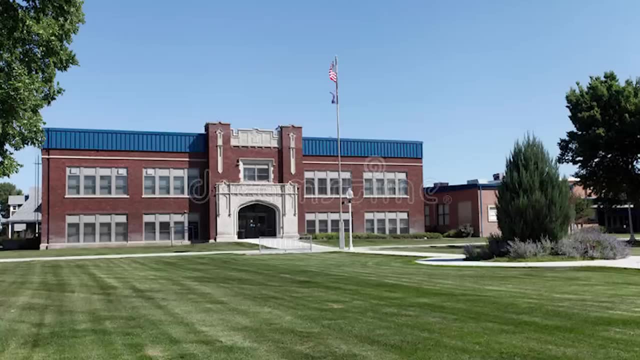 you aren't catching up. There was one time I was sick with a fever. My head was so hot you could probably cook your breakfast on there. I had to take a week off and when I came back to school I saw this. 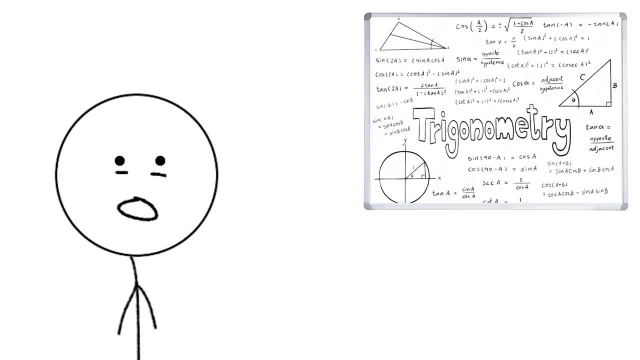 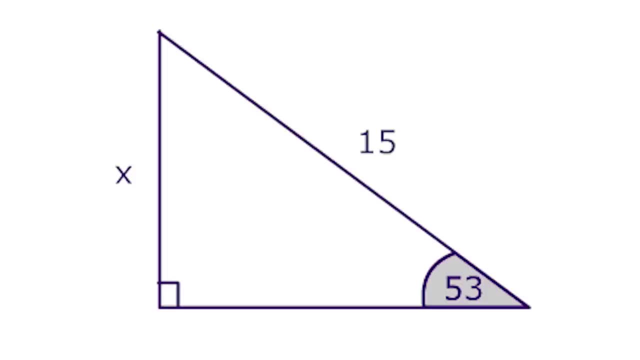 You know what My fault? I should have just stayed at home. There seems to be an obsession with triangles sine cosine tangent. Now I get it. you can find the length of this side using these two, or you can find the. 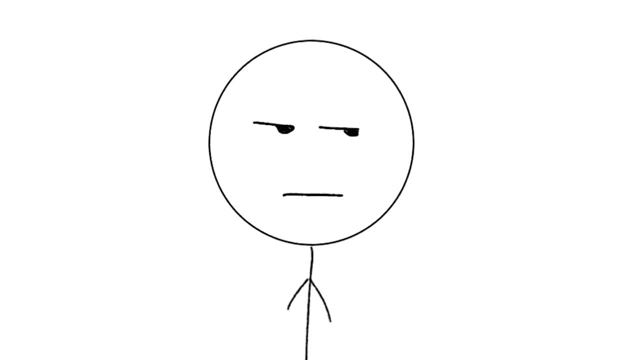 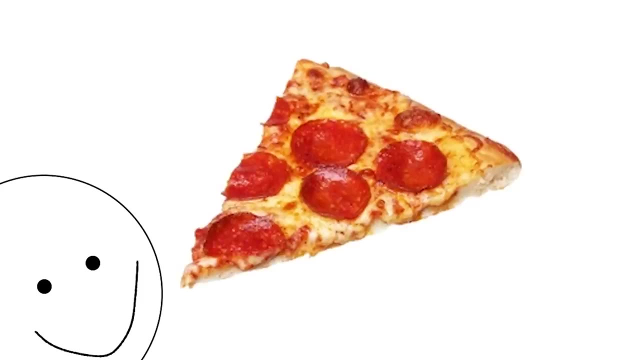 angle of this, using these two Right, so don't get me wrong. I can appreciate the look and taste of a Dorito or the appetizing allure of a slice of pizza. I can even appreciate the aerodynamic efficiency of that yellow angry bird that goes fast. 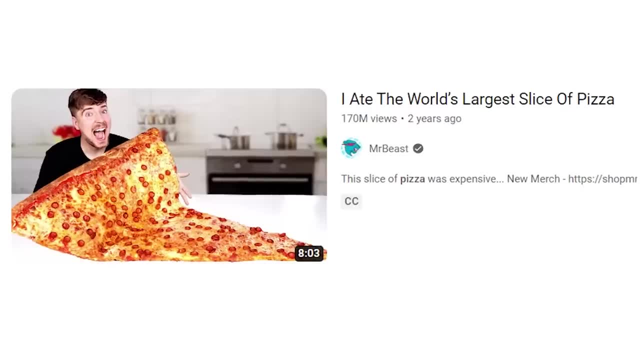 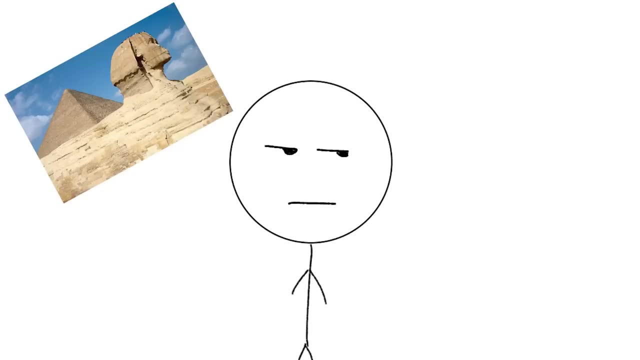 And listen. if I'm trying to be the next Mr Beast making a bigger slice of pizza, or if I was in ancient Egypt making pyramids, I'm all ears. But we're not in ancient Egypt, we're not making pyramids and I need to cut down. 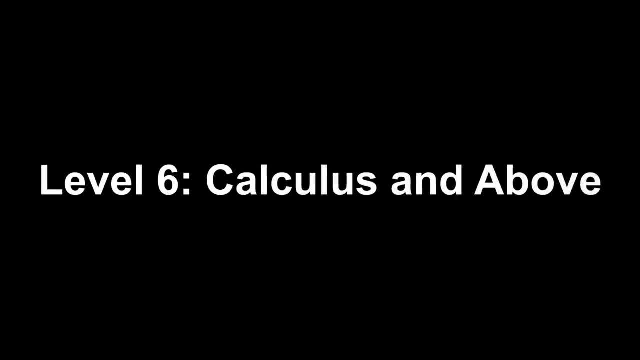 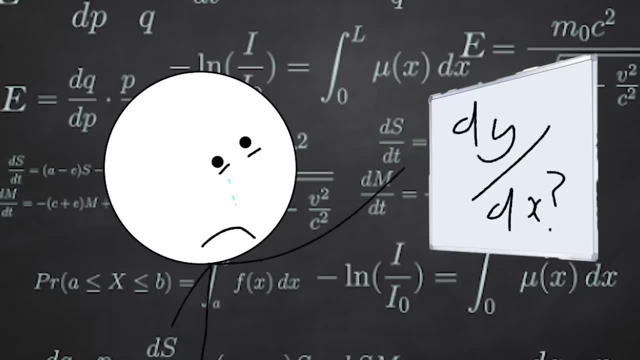 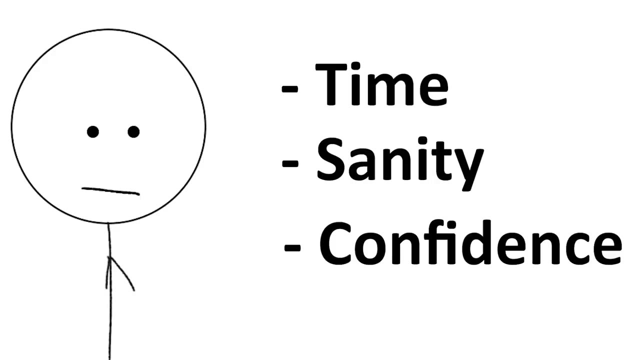 my consumption of pizza, not increase it. Level 6, calculus and above. To anyone who was unfortunate enough To undergo the insufferable topic that is calculus, first of all, I am sorry for your loss. The loss of time, sanity and self-confidence is something that will never get back. 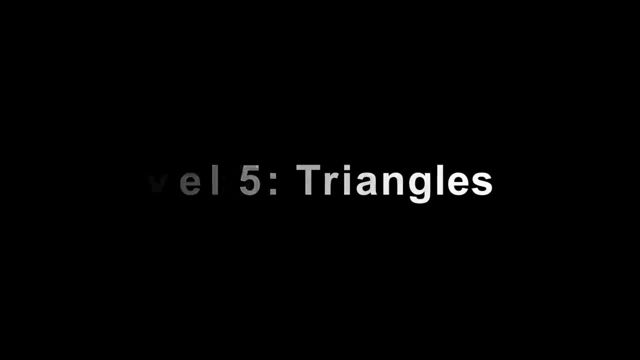 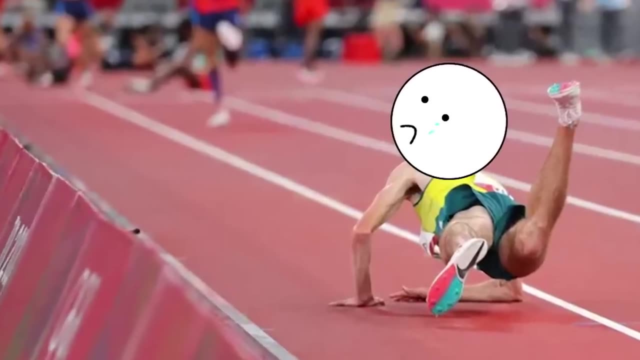 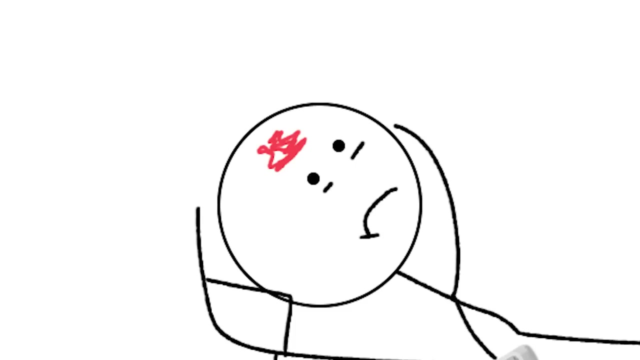 Level 5, triangles. I remember in the final stages of secondary school. if you miss a class it's game over, Just like tripping over at the start of a 100 meter sprint: you aren't catching up. There was one time I was sick with a fever. My head was so hot. 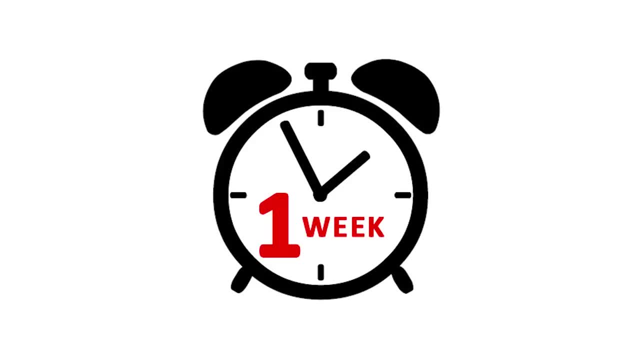 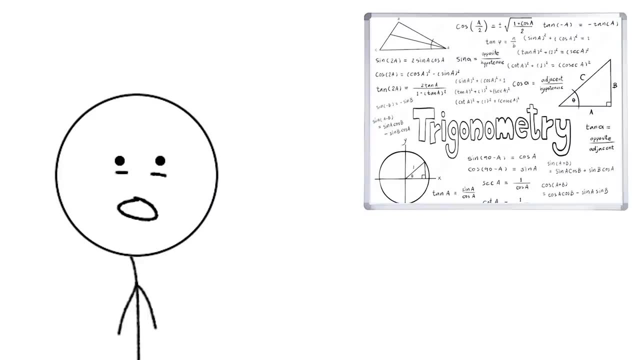 you could probably cook your breakfast on there. I had to take a week off and when I came back to school I saw this. You know what My fault? I should've just gone to school. I should've just gone to school. I should've just gone to school. I should've just. 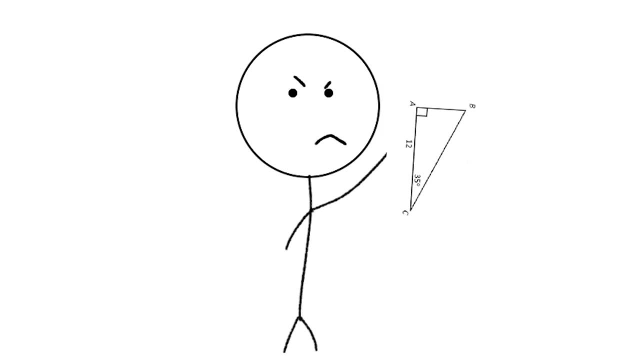 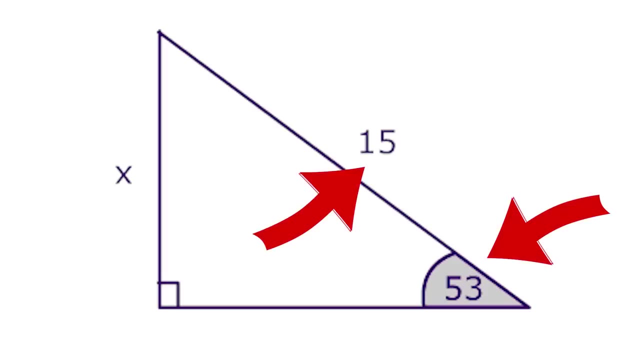 stayed at home. There seems to be an obsession with triangles, Sine cosine tangent. Now I get it. You can find the length of this side using these two, or you can find the angle of this using these two Right. so don't get me wrong. I can appreciate the look and the taste of a Dorito. 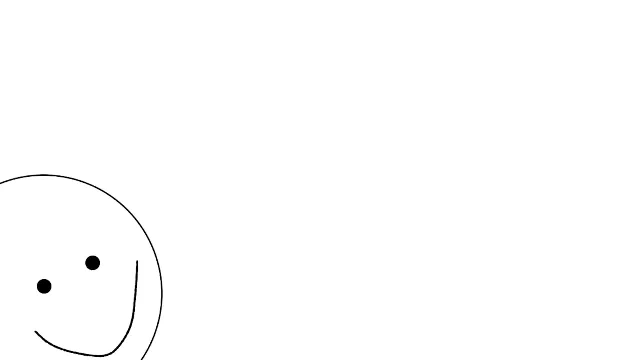 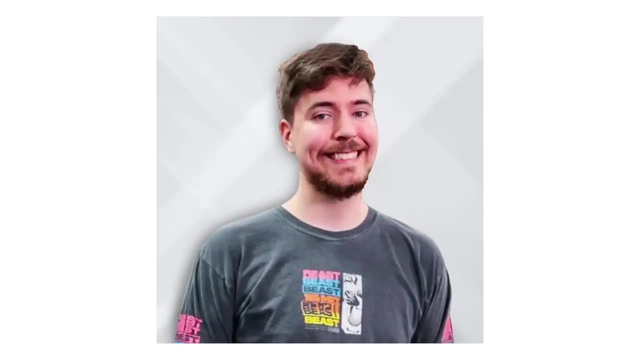 or the appetizing allure of a slice of pizza. I can even appreciate the aerodynamic efficiency of that yellow angry bird that goes fast. And listen if I'm trying to be the next Mr Beast making a bigger slice of pizza, or if I was in ancient Egypt making. 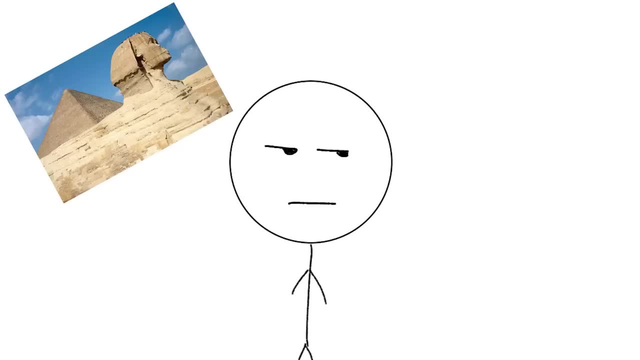 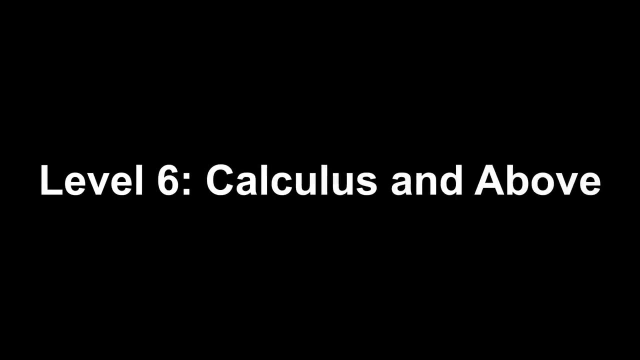 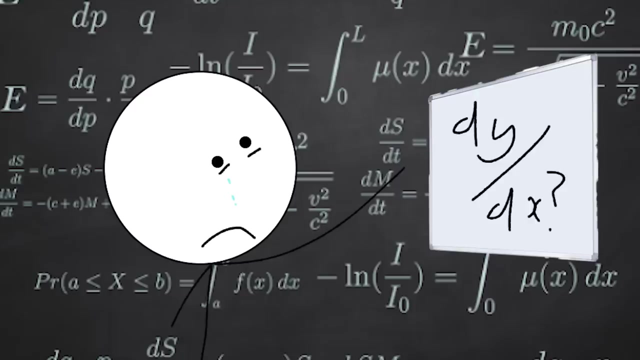 pyramids. I'm all ears, But we're not in ancient Egypt, we're not making pyramids, and I need to cut down my consumption of pizza, not increase it. Level 6. Cackless and above. To anyone who was unfortunate enough to undergo the insufferable topic that is cackless: 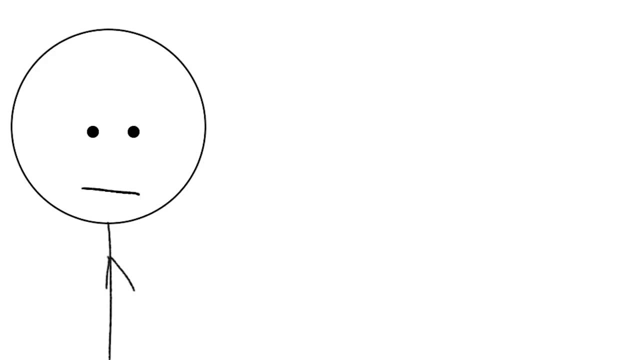 first of all, I am sorry for your loss. The loss of time, sanity and self-confidence is something that will never get back. Cackless is seen as the final boss in math and for a topic that is meant to derive, I feel that it derived nothing but a slight. 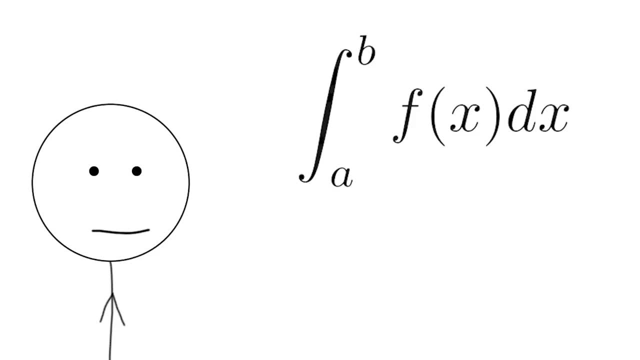 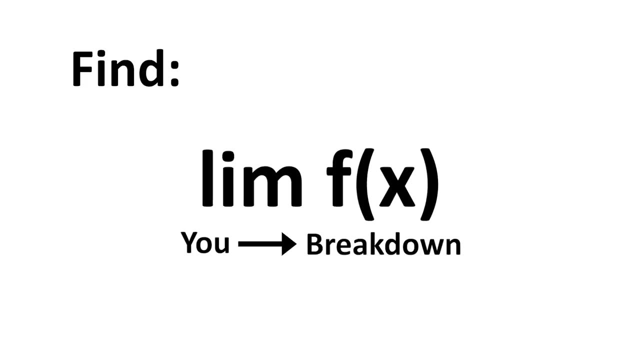 loading for math as a whole, And the only integration it had achieved was that of a collective resentment for math. Cackless taught us to find our limits as we approached a breakdown, and also it taught us to never trust titles on YouTube videos. But after reading the comments. 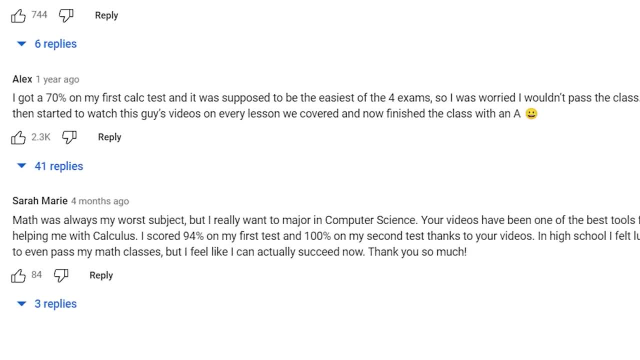 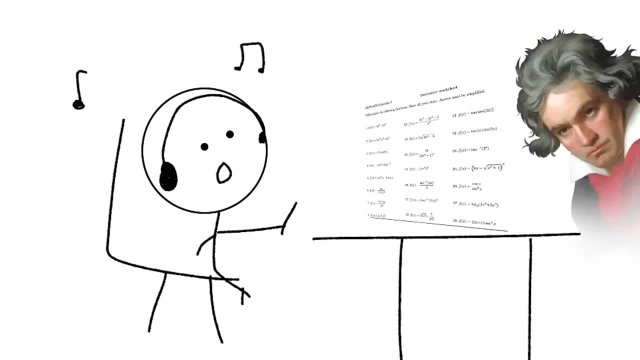 praising how it helped them with their grades. you sit there questioning if it's a me problem After countless hours of studying with classical music, playing, thinking it'll make you smarter. something clicks in your brain, making you feel like a genius for getting a question right. 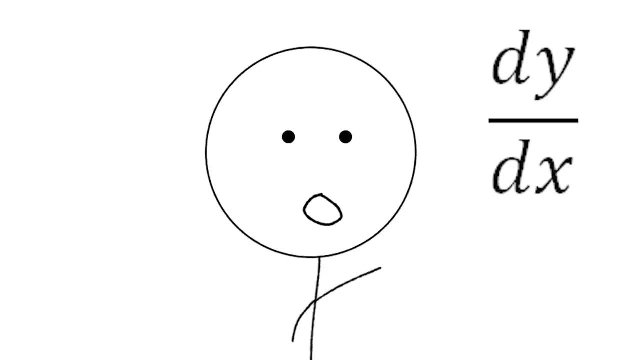 Calculus is seen as the final boss in math and for a topic that is meant to derive, I feel that it derived nothing but a slight loading for math as a whole, And the only integration it had achieved was that of a collective resentment for math. 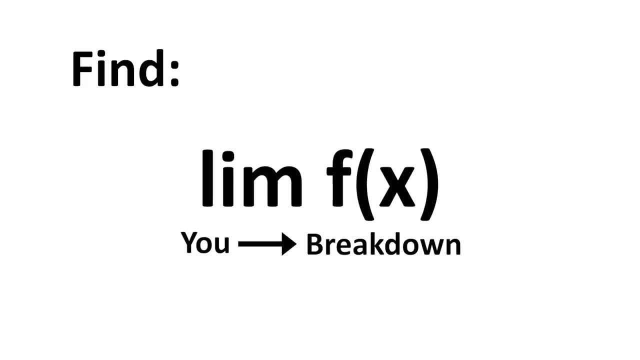 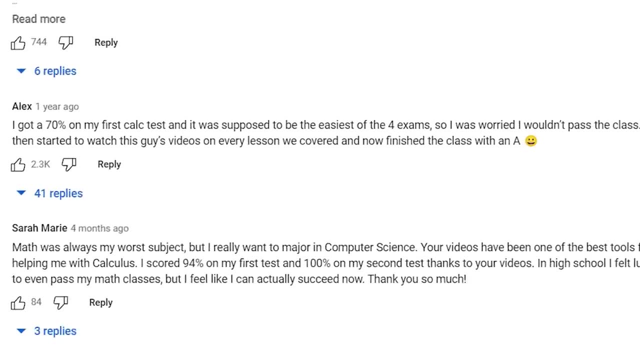 Calculus taught us to find our limits as we approached a breakdown, And also to find our limits as we approached a breakdown. It taught us to never trust titles on YouTube videos. but after reading the comments praising how it helped them with their grades, you sit there questioning if it's a me problem. 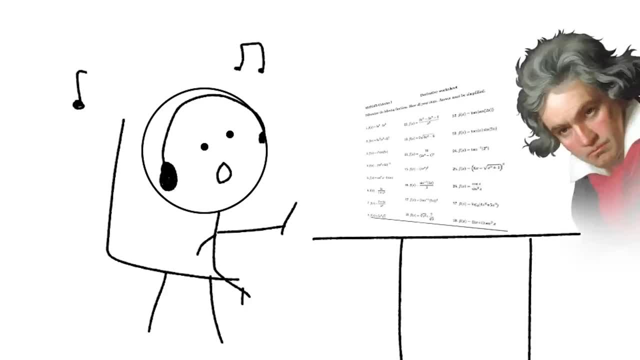 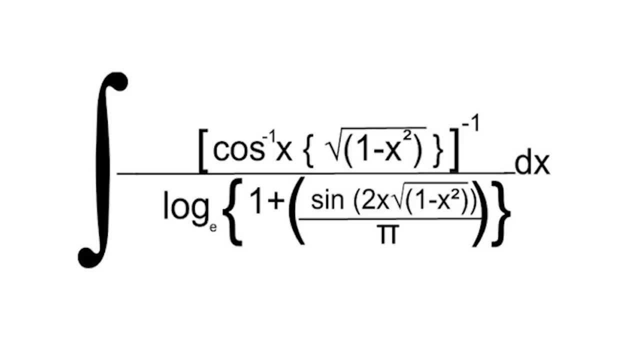 After countless hours of studying, with classical music, playing, thinking it will make you smarter, something clicks in your brain, making you feel like a genius for getting a question right. But for the harder questions, you write random letters and numbers, hoping it's right. 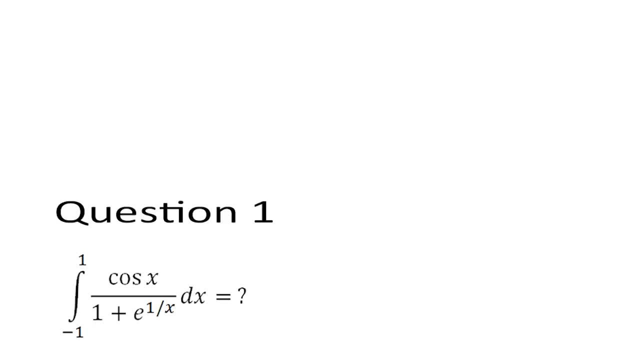 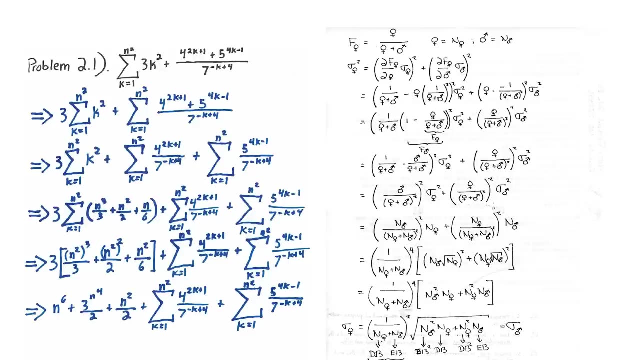 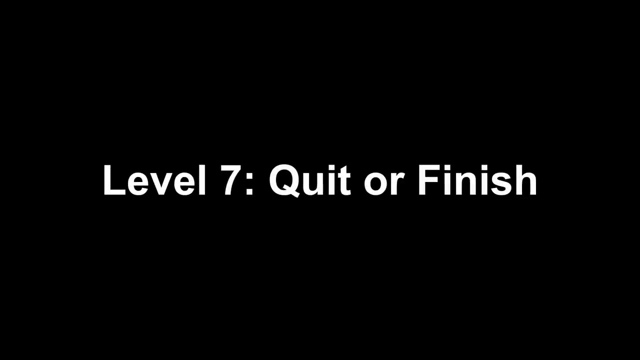 But if it's one of those extended questions where a question is based on a previous question, you sit there and accept the fate of a bad grade. Eventually, after many repetitions of what seems like the worst human experience possible, you move on to level 7.. Level 7. Quit or Finish. 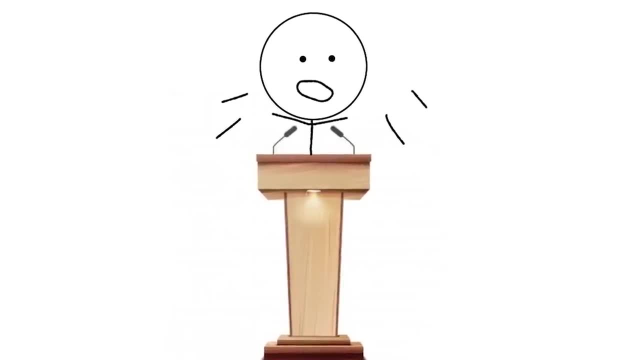 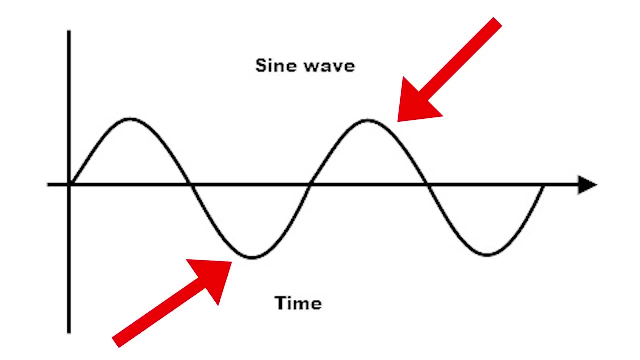 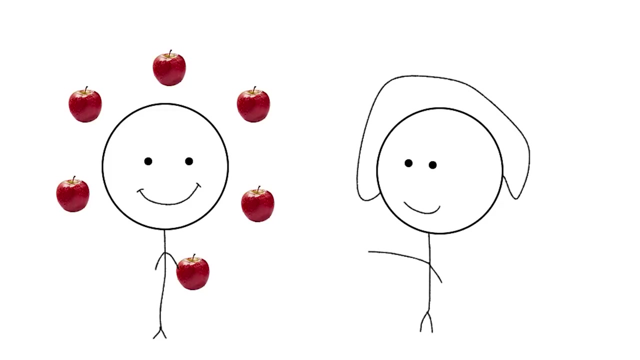 After a long journey exploring a glimpse of what mathematics has to offer. level 7 is the end of learning math, at least from an academic standpoint. The highs and the lows, The late nights and early mornings: What was it all for? We started off deciding how many apples we should share. 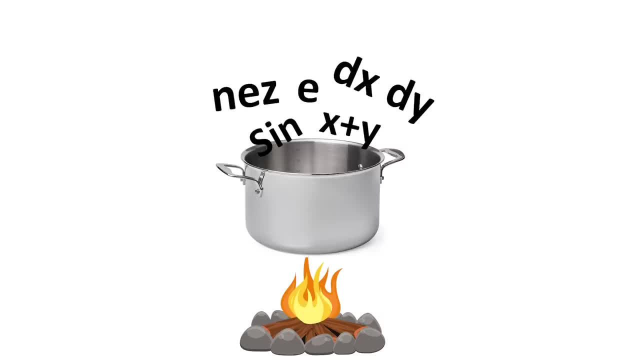 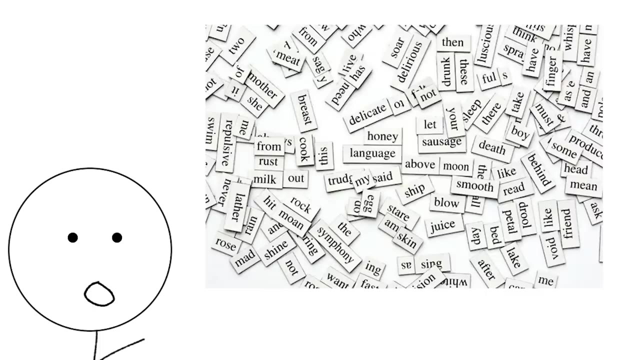 and quickly descended to cooking an unsavoury mix of simple soup. Something I noticed I was asking myself often when learning math was why? Yes, the instinctive answer is to get good grades, but it often felt like the topics in math had no utility in our immediate lives. New words learnt in English can be applied in the world. 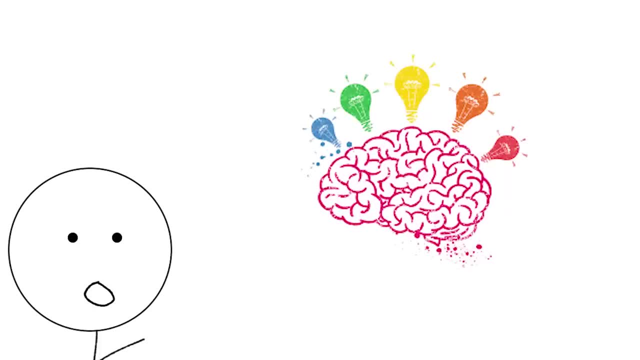 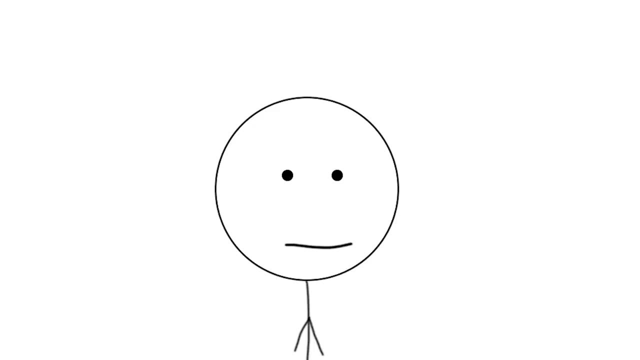 outside of exams, and even things that can't be applied physically, such as the concepts learnt in science, gives us some sort of understanding of the world of the future. This can be applied of the world In the case with mathematics, excluding the fundamental skills discussed. 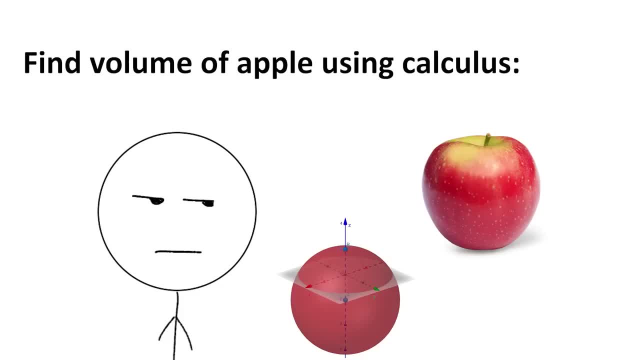 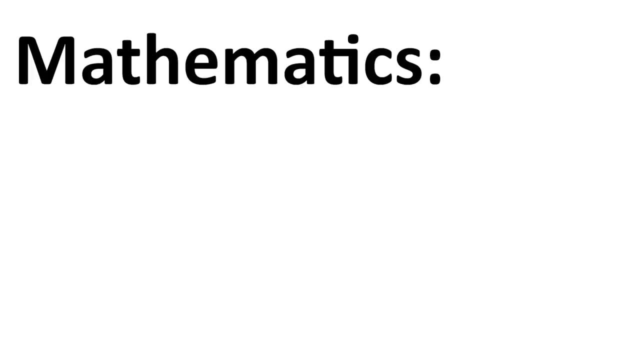 in the earlier levels, the ability to apply what we've learnt in a meaningful way seems to be limited. We were taught to solve for y, but didn't know how to solve the y. But with a subject with so many problems and depending on us to solve them, it was a red flag from the beginning. 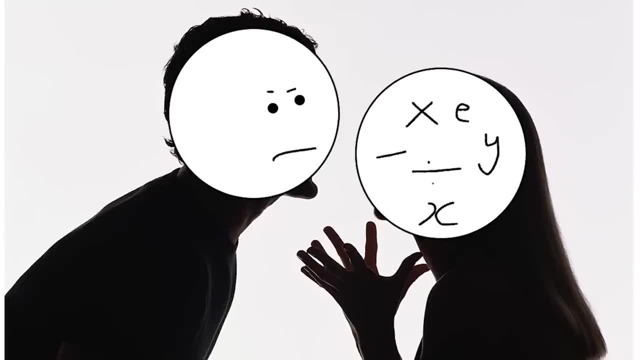 And with most of the world requiring students to study mathematics, it seems like a toxic relationship forced upon us. Thank you for watching.